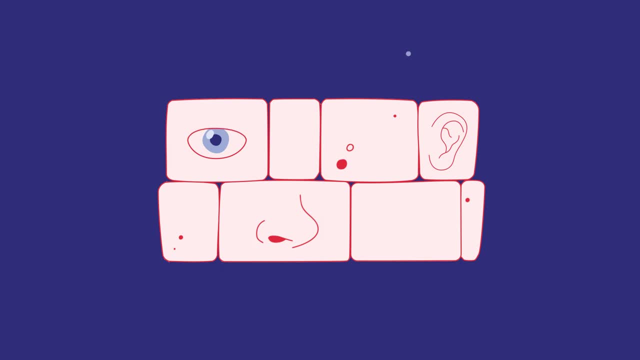 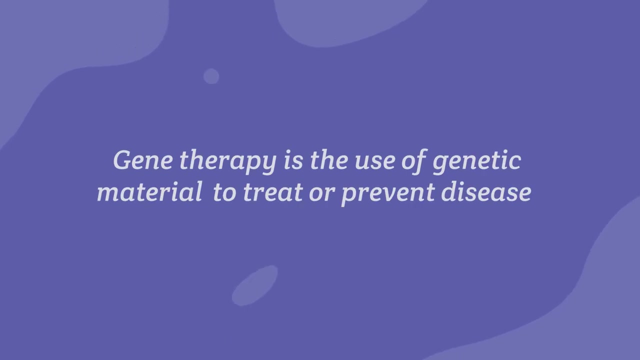 That's where gene therapy aims to help by addressing the underlying cause of disease. If genes are like the blueprint to our body, gene therapy can fill in missing parts or correct errors in the drawings. Gene therapy is the use of genetic material to treat or prevent disease. The genetic material used or targeted is DNA or RNA. 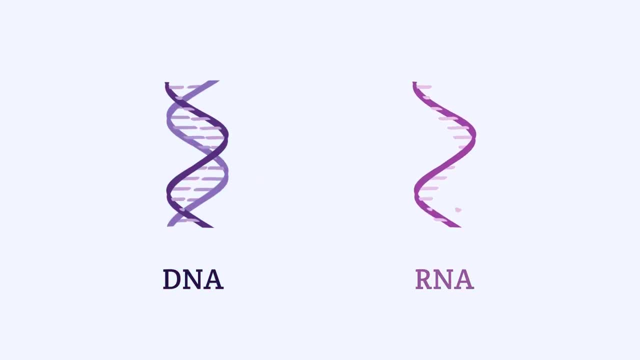 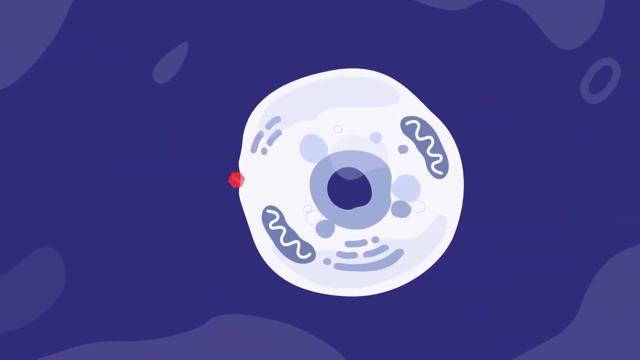 DNA stores our genetic information, whereas RNA is a modified copy of that information needed for the cells to build the correct protein. In gene therapy, the genetic material is used to. The genetic material is transferred to the cells and then changes how proteins are produced by the cell. 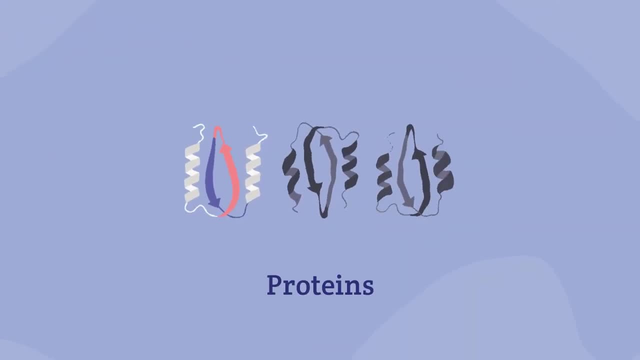 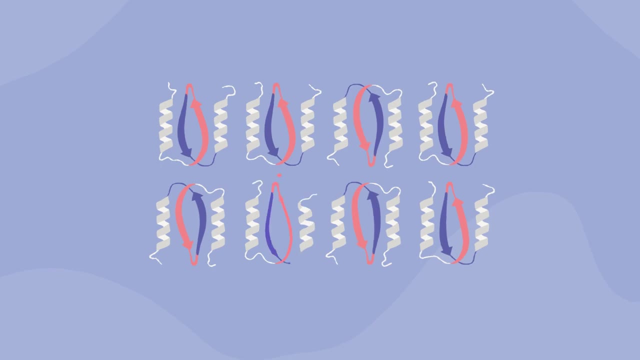 It can reduce levels of certain disease-causing proteins, increase production of working proteins or even produce new or modified proteins within the cell. The genetic material needs help to get where it needs to go, like being wrapped in a package with an address label. 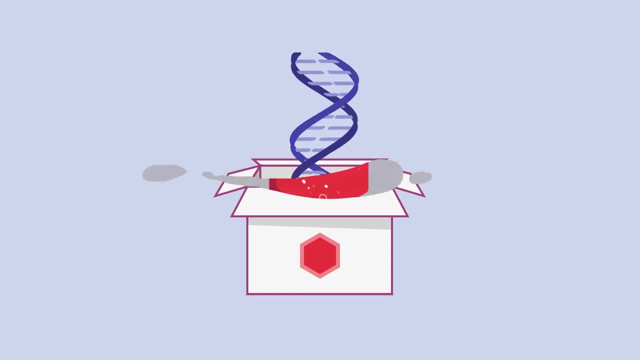 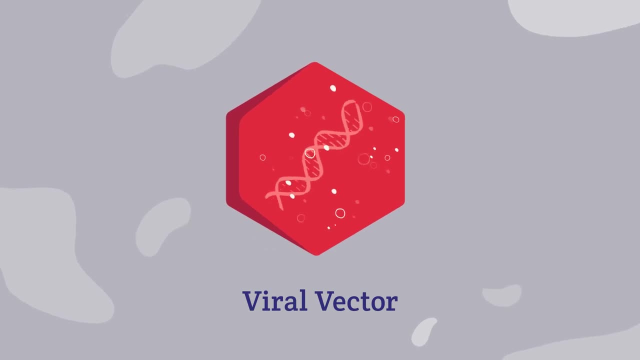 This package delivering the genetic material is known as a vector. Typically, viruses are used as vectors because they've evolved to be very good at getting into cells, But in this case, scientists use this same ability to deliver the new therapeutic genetic material into the cell. 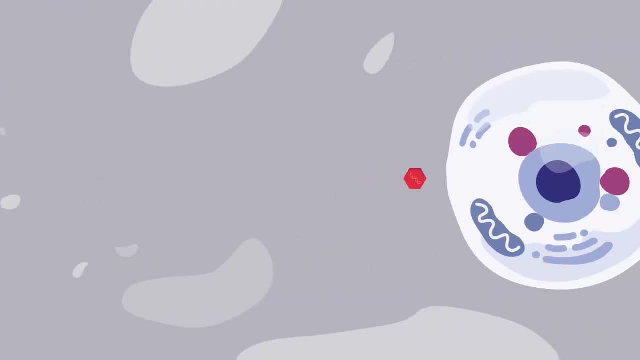 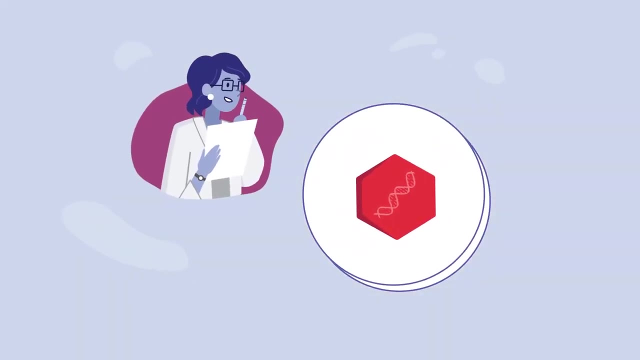 Any disease-causing part of a virus is removed, allowing it to enter the cell without making a person sick. All vectors are tested many times for safety prior to being used in humans. There are two main ways to give gene therapy: In vivo and ex vivo. 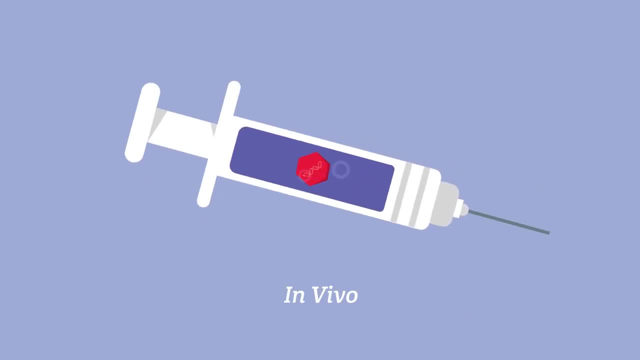 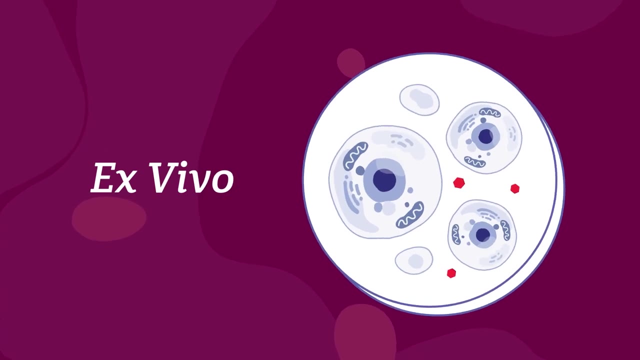 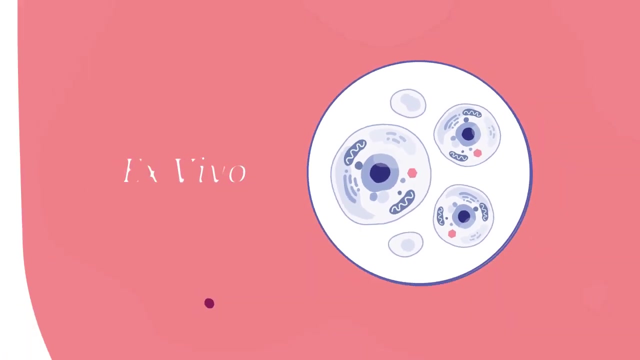 In vivo gene therapy means the gene is delivered directly into the person, such as through an injection. Ex vivo gene therapy removes the person's own cells and delivers the gene to these cells outside the body. These modified cells are then returned to the person. 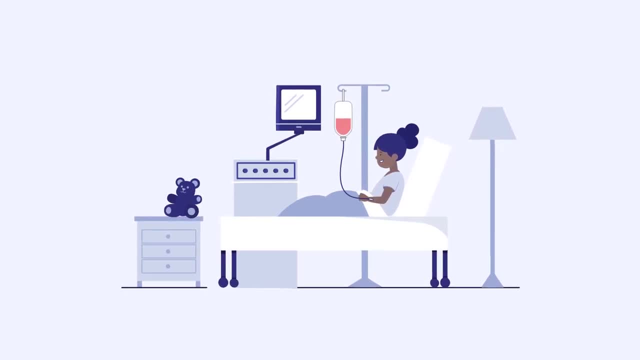 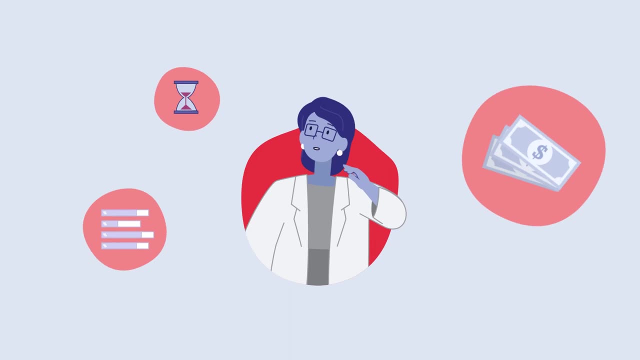 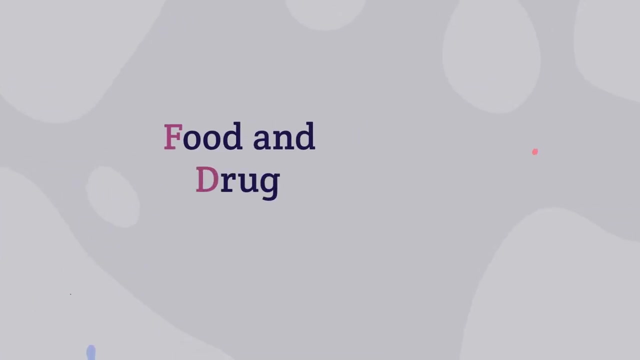 Deciding the right approach depends on the best way to target the disease. There are still many challenges to be overcome. There are still challenges to overcome for those seeking gene therapy as potential treatment options. One challenge is time. It's a lengthy process to test potential treatments in clinical trials and then undergo 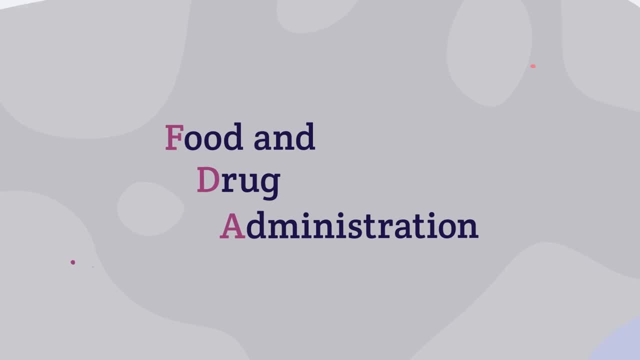 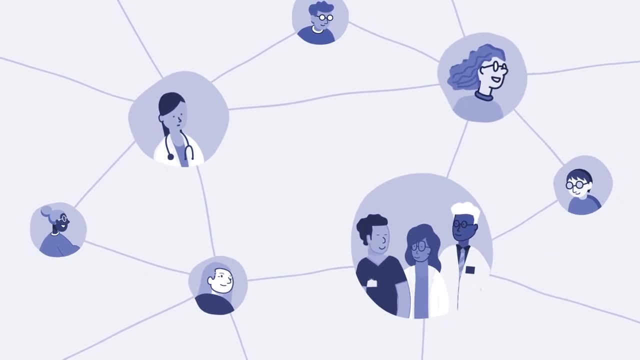 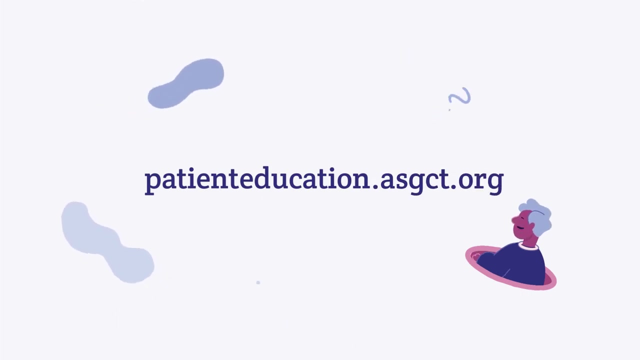 the FDA approval process, But advances in gene therapy research allow us to better understand how we could treat, and hopefully someday prevent, rare and debilitating diseases. For more information and resources about gene therapy and how it works, go to patienteducationasgccom, gctorg.